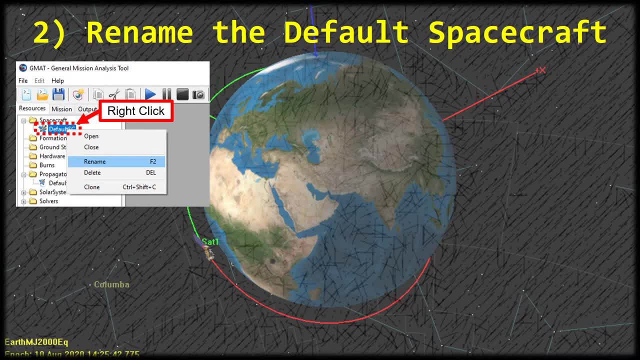 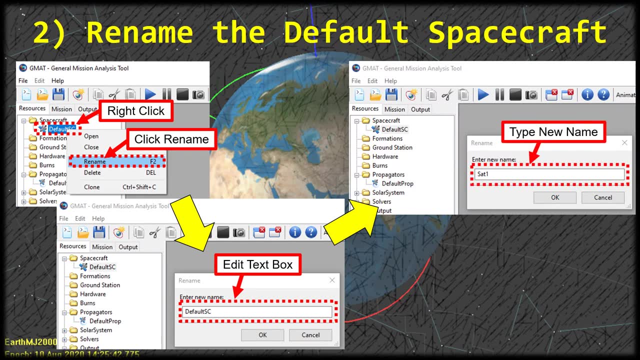 when you right click on that, you'll see the menu pop up and we're going to click rename and that's going to open up this window here with an edit text box. We're going to type in the new name And so let's just go ahead and call that SAT1 for space. 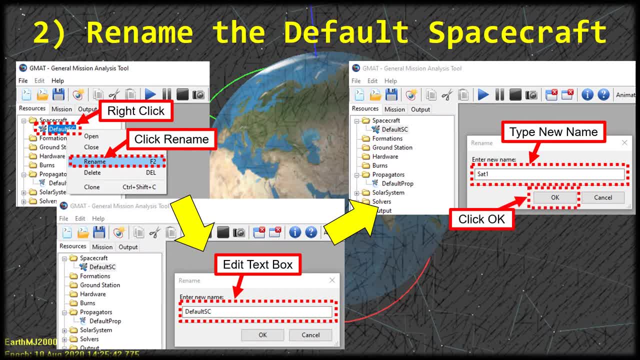 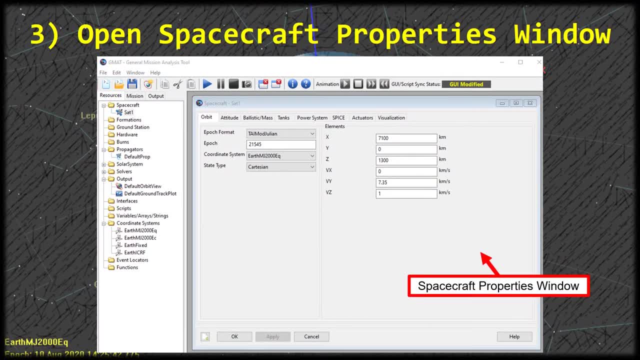 Satellite 1.. So type that in the box and click OK. Now that we renamed the satellite, let's go ahead and open up the spacecraft properties window. You can do that by double clicking on the object in the left project viewer window. We renamed it SAT1,, so find SAT1 and double click on it With the properties window open. 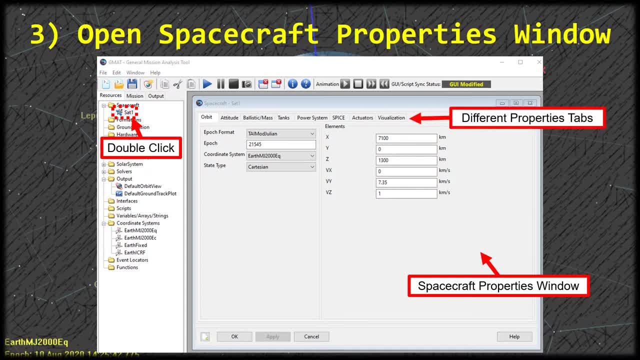 you'll notice that it has a bunch of tabs at the top. Each of those tabs have a group of properties. For this tutorial we're going to just focus on a simple orbit, And so we're going to stay here on the orbit tab and adjust those parameters. only In future videos we'll cover some of 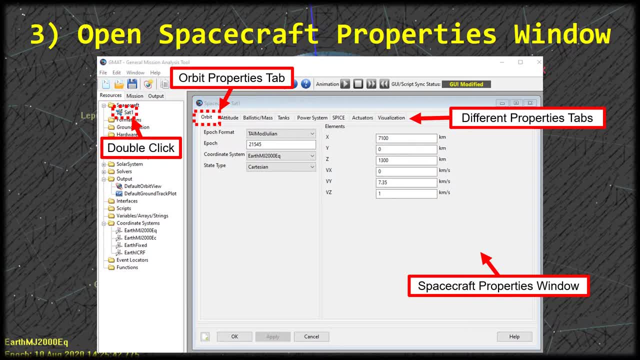 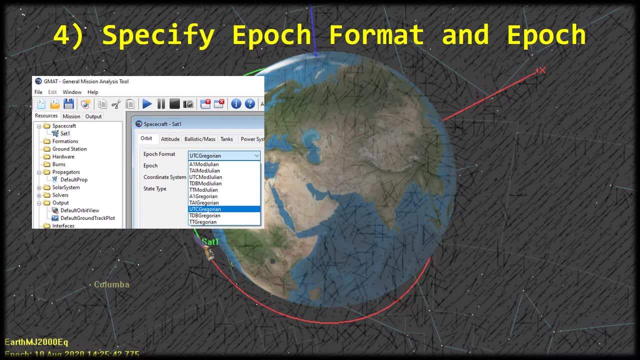 the other tabs and properties in those tabs. Let's get back to the tutorial and entering in the orbital elements. As a reminder, we're on the spacecraft properties window for SAT1.. We're first going to start with specifying the epoch format and the actual epoch. 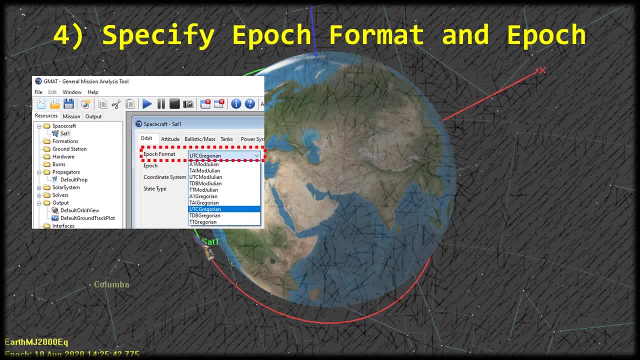 On the orbit tab. if you look on the left, the first selection box gives you the option to choose the format that you want to specify the epoch. For our tutorial we're going to use UTC, Gregorian, So find that in the list and click on it With the format specified. 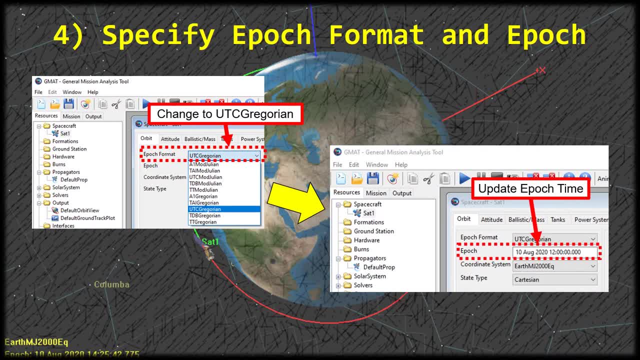 we can go ahead and actually enter in the epoch time Now for UTC Gregorian, it's very important to get the format right. This basically takes the text entered into epoch and breaks it up into the different pieces. If you get the format wrong, it's going to have an error And it will tell you if you. 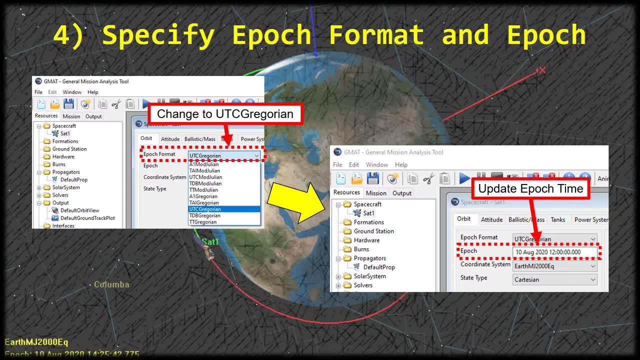 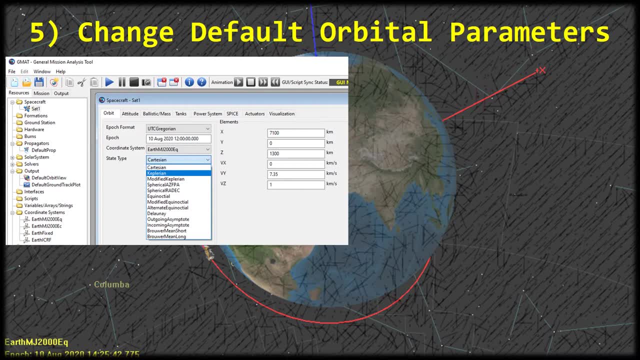 entered it in incorrectly. So go ahead and choose your epoch time. Moving on to the other orbital parameters or orbital elements, You'll notice that the default state type is Cartesian. We're actually wanting to specify our orbit using Keplerian, So in the selection box for state type, go ahead and find Keplerian and select it. You'll. 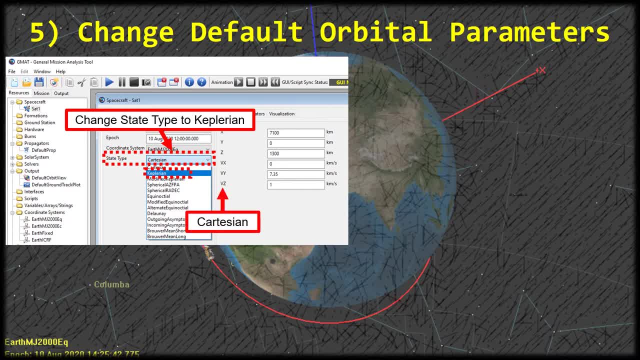 see that the values in the right column change from Cartesian Elements and Format. You'll see that the values in the right column change from Cartesian Elements and Format. You'll see that the values in the right column change from Cartesian Elements and Format. 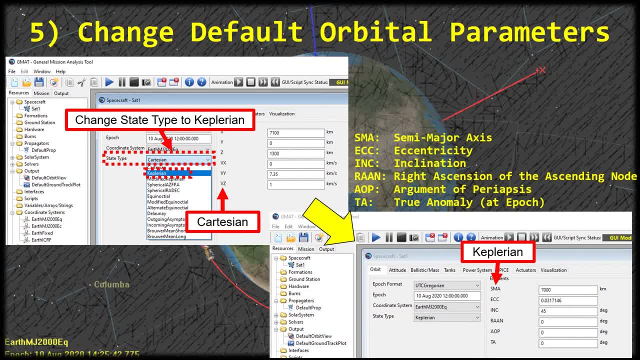 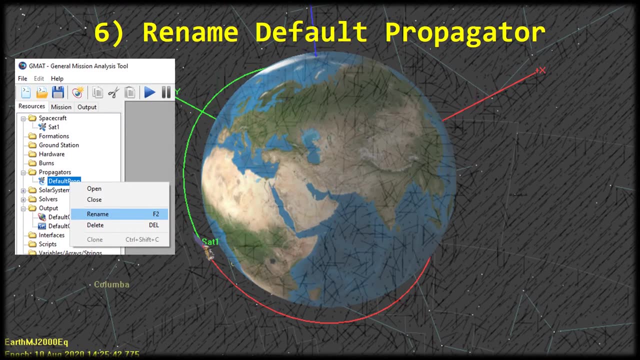 And, as you can see, they have the units there on the right of the box, so you know which units to use. So go ahead and fill in the orbital parameters and then, when you're done with that, click OK. With that, we're done editing the spacecraft properties. Let's move down and start editing. 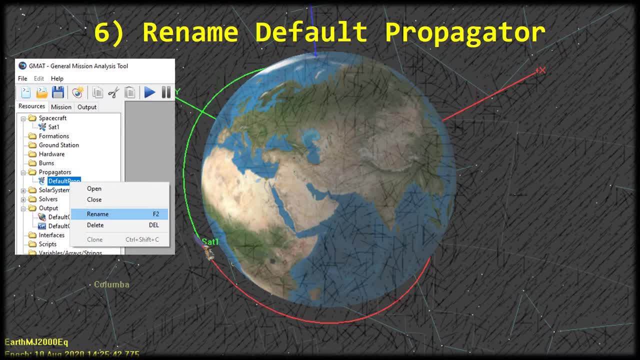 the default propagators properties. We're first going to change the name of the default prop. So in the tree on the left, If the propagators folder is minimized, go ahead and click on the plus sign next to it to expand it out so that you can see the default propagator. Right click on it and then in the menu that. 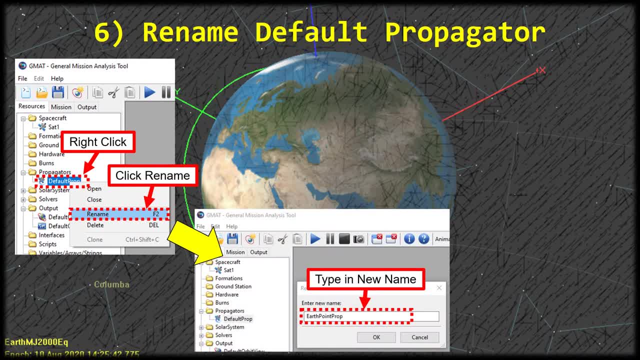 appears, go ahead and click rename. That will open up a window with a edit text field where you can type in the new name. I'm going to go ahead and call this one an earth point prop. So when you typed in the new name, go ahead and click okay and you'll notice in the tree on the left that 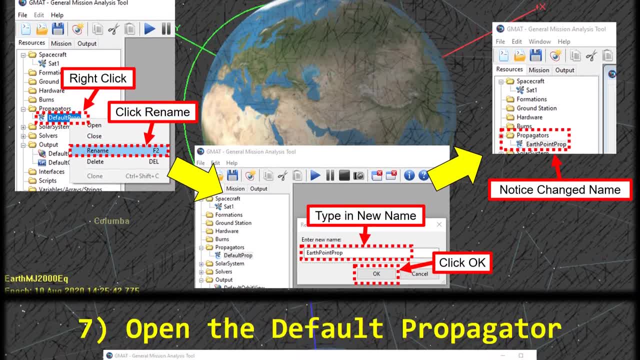 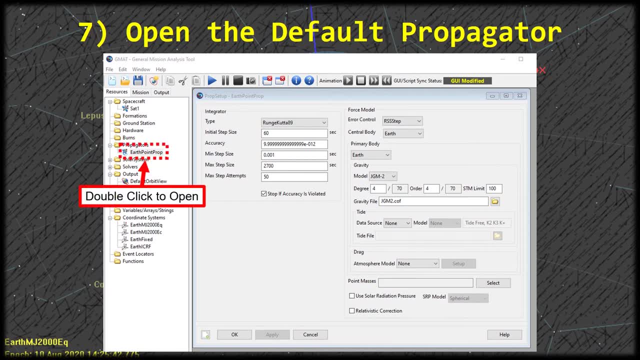 the name has been updated, So now we're going to go ahead and double click on it in the tree view to open up the propagator properties window. This window is split into two columns. The first column contains different variables or settings for the integrator of the propagator, and the second 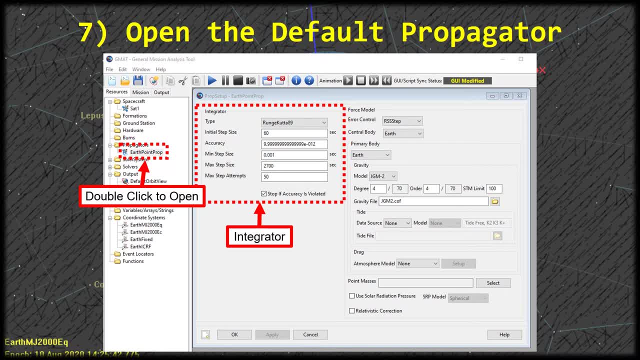 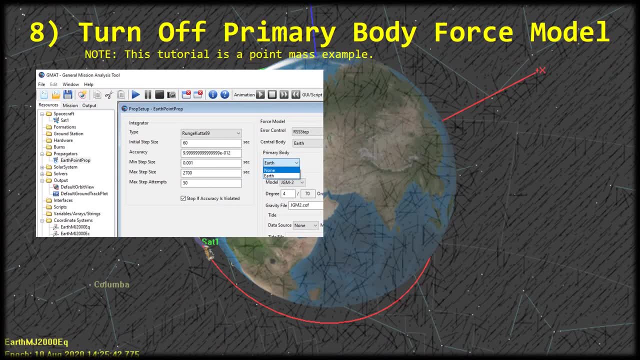 column contains the parameters or variables or settings for the force modeling that GMAT does For this example, I'm going to go ahead and click on the plus sign next to it to open up the new name. In this tutorial, we're going to leave the integrator properties alone and just let it. 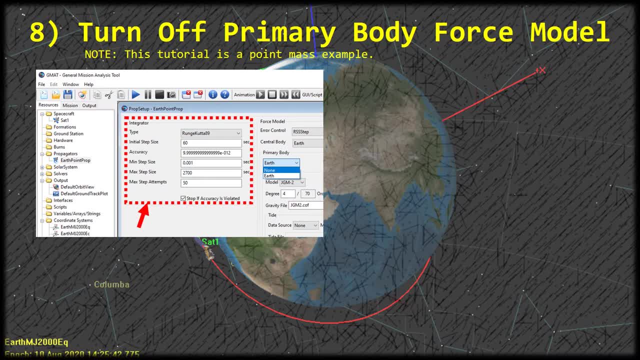 use the default values. We're also going to leave the central body on earth, because that's what we want. to orbit around, However, we do need to change the primary body from earth to none. This is because we are doing a point mass example and we don't want to have, or rather we don't care about. 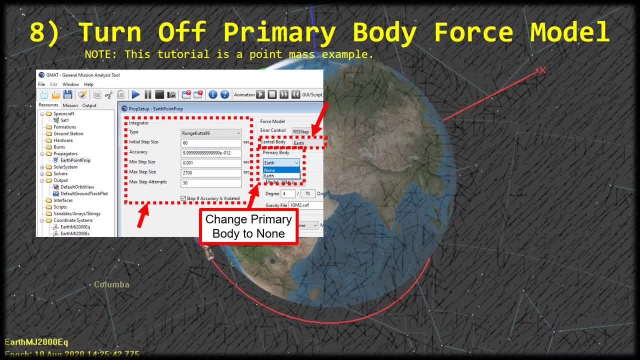 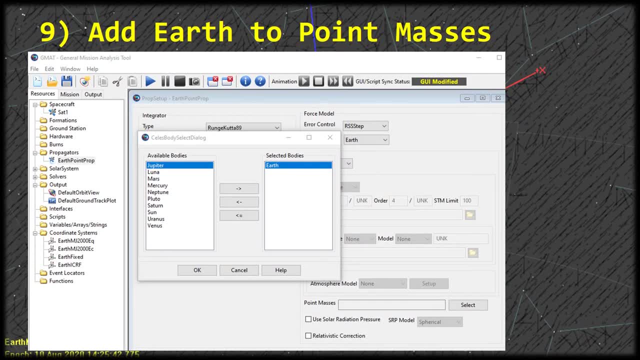 a gravity model or a drag model. So when you click none, you'll notice that the gravity and drag models get greater. So we're going to go ahead and click on the plus sign next to it to open up the integrator. Now we need to add earth to the list of point masses that the propagator, or rather force. 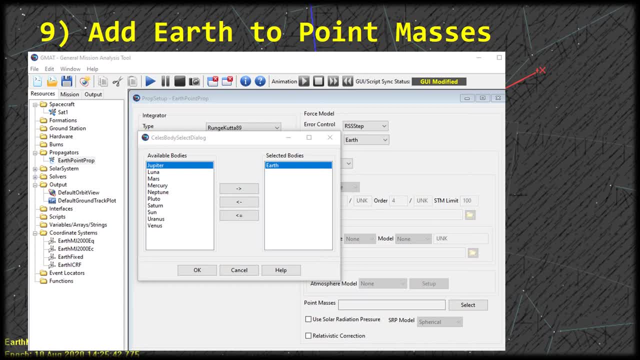 model takes into account, And the right hand column towards the bottom, you'll notice that there is a button that has the label select on it, next to the point masses area. If you click on that, it will open up this window. This window is used to specify which of the available bodies you 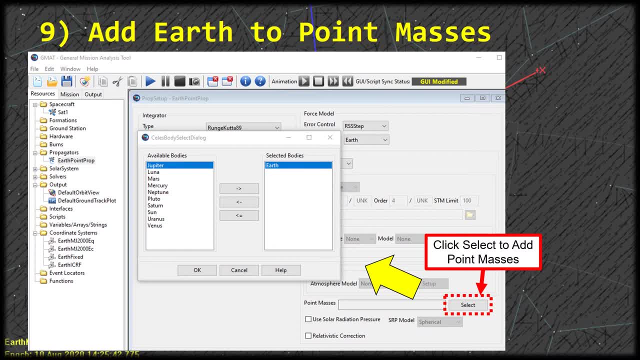 want to use as a point mass. in your example, To use something out of the list of available bodies in the point mass force modeling, we need to move it from the available column to the selected column. So to add a body to the model, we need to find it here in the left column and then click this. 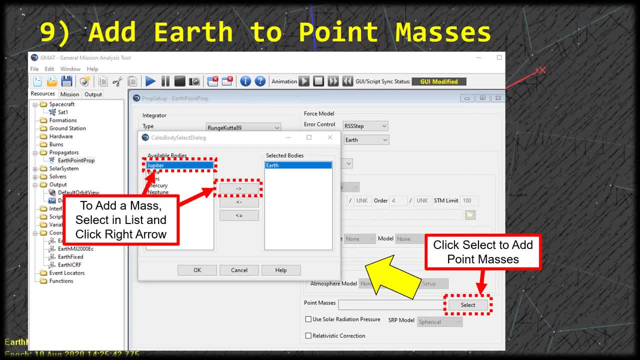 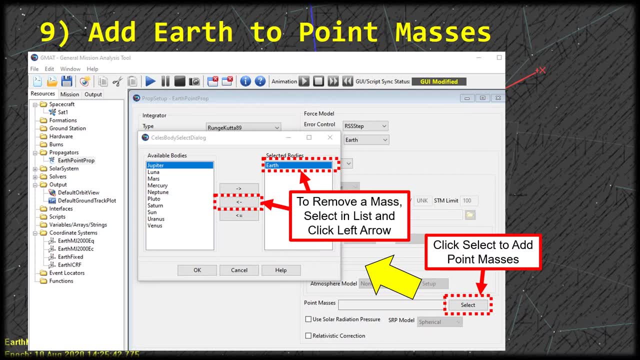 top button, which is a right arrow, to move it from the available bodies to the selected bodies. If we wanted to remove a point mass from our force model, we would select it here in the right column, in the selected bodies column, and then click the left arrow to move it back into the available bodies. 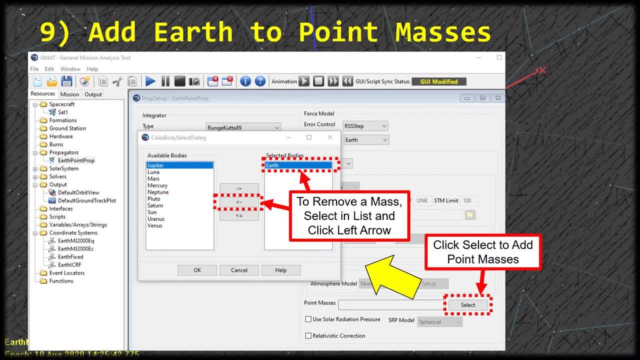 list. In this tutorial we're just going to have earth as our point mass, So select earth and deselect anything else that might already be in the selected bodies column And when you're done with that, go ahead and click OK. When you do that, you'll notice that the point masses that. 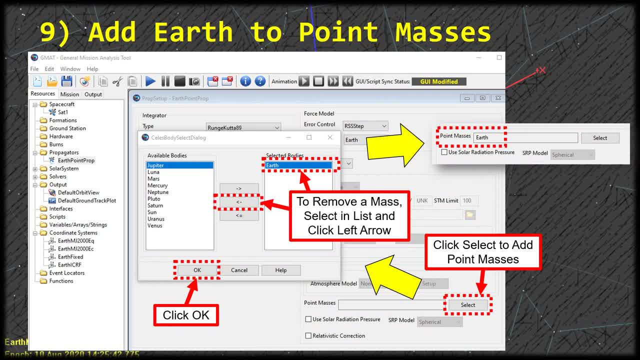 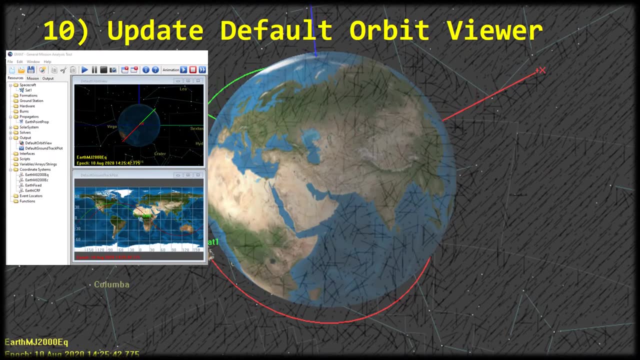 is being modeled shows up in a list next to the button that you clicked to open the window. And that's going to be it for the propagator. So go ahead and click OK on this window to save the changes to the propagator. The default object has two other output objects that will appear when we actually run the project. 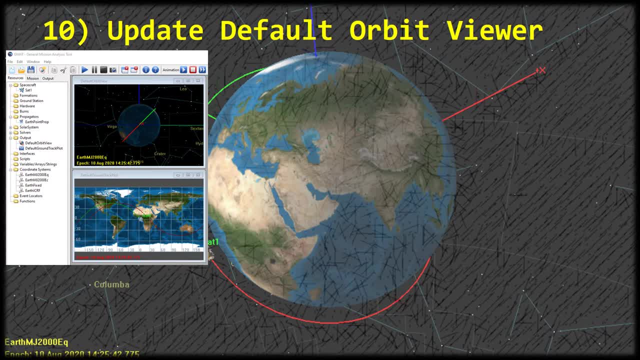 I show them here on the left. The orbit view is a 3D modeler that allows us to zoom in, zoom out, allows us to pan or rotate to get a better view of the body. we're orbiting of the object. we're orbiting of the object. we're orbiting of the object. we're orbiting of the. 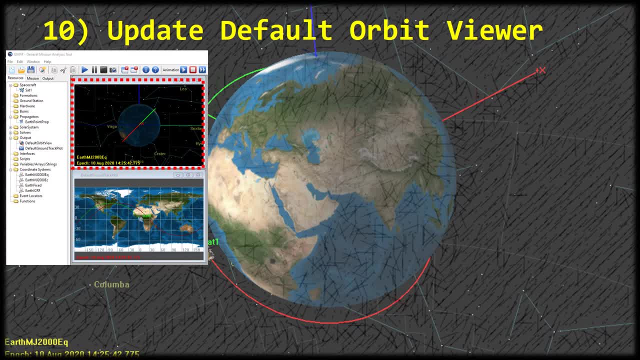 body that is being orbited of the orbit path. It also allows us to hit, play and see an animation of our project. The bottom one is a ground track plot that allows us to see how our satellite flies over the earth. We're going to update some of the properties of the orbit viewer, the top one here. 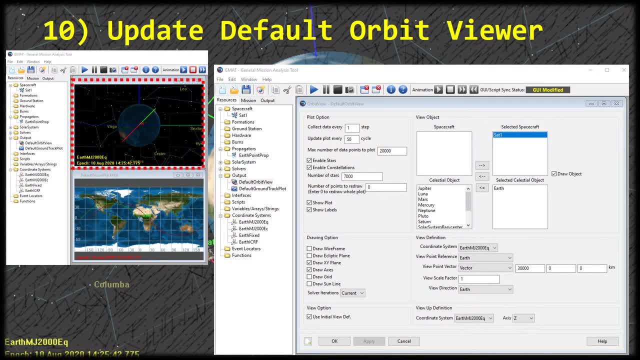 So in the tree on the left under the output folder, if you expand that, you should see a default orbit view. Go ahead and double click on that and that will open the object. Open up the properties window for that object and you'll see this window. There's a lot going on. 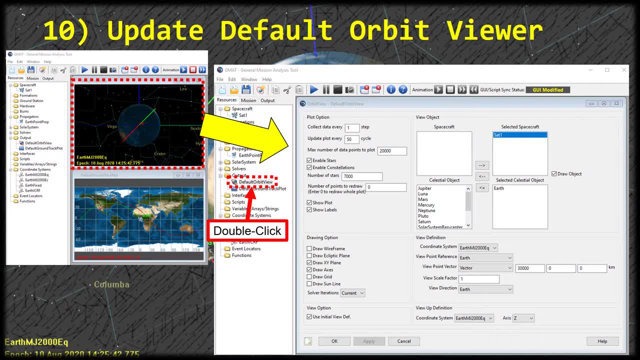 in this window and it's all about making that orbit viewer. We have different options for how we plot things. We have different options for what objects we view or where we view from. This would be adjusting the camera, along with some other drawing options. So let's go ahead and on the 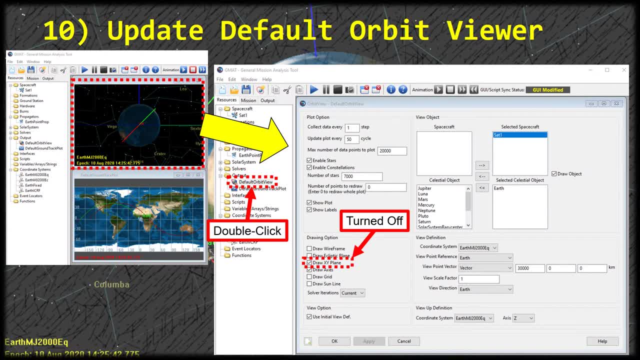 left column. we're going to go ahead and turn off the XY plane. You don't really need to do that, I just think it looks better with it turned off. So let's go ahead and turn off the XY plane, At least with earth. We're also going to go to the top right and adjust what objects we view. 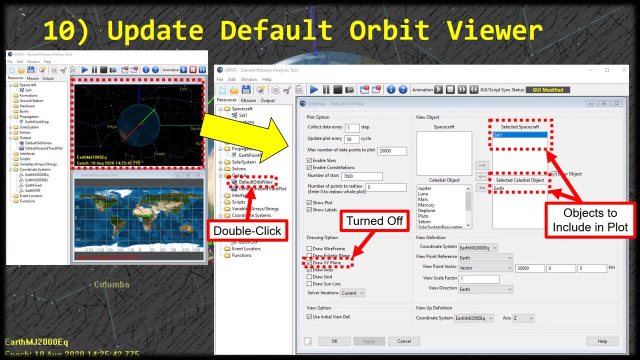 Of course, we want to make sure that the spacecraft that we're actually doing this project for is shown in this. So go ahead and make sure our spacecraft, or sat-1, gets moved from the list of available spacecraft into the selected spacecraft. Likewise, we're going to go ahead and include 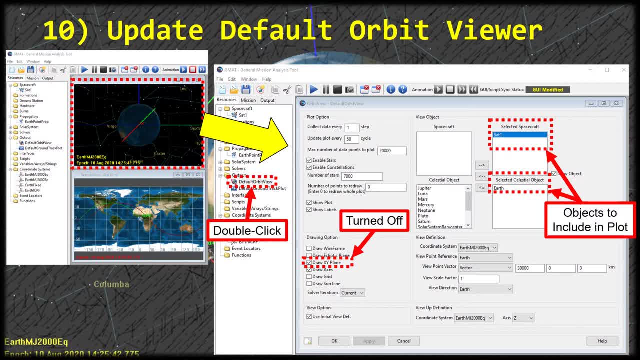 earth as a plotted celestial object. You can add other ones in there if you want to, but we're just going to do earth for right now And then we're going to go ahead and select the object that we're going to view right now And then click OK. when you're done with that, In a later video I'm going 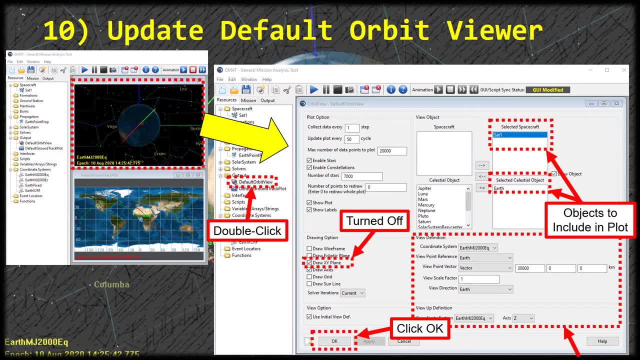 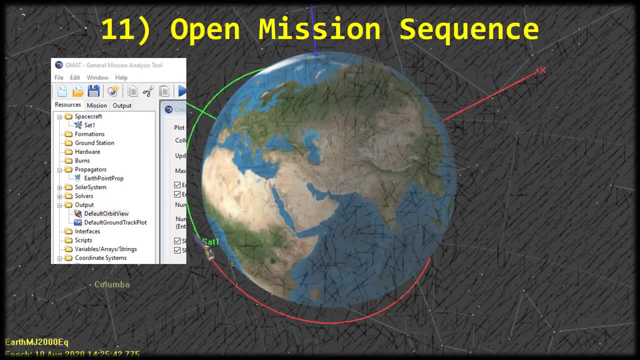 to go ahead and talk about the view definition and how we can move the camera around to see better shots of the orbit. So stay tuned for that video. Up to this point, we've been working on the resources tab, which allows us to add objects and modify their properties. However, now we're going. 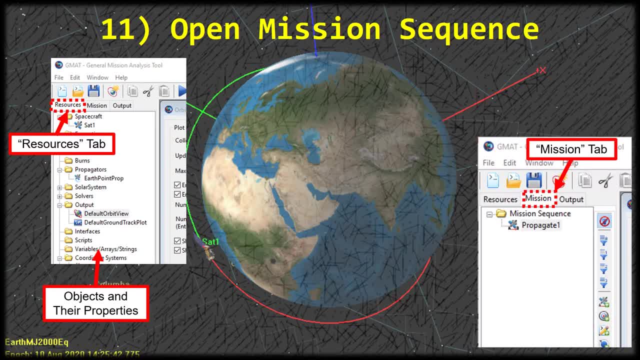 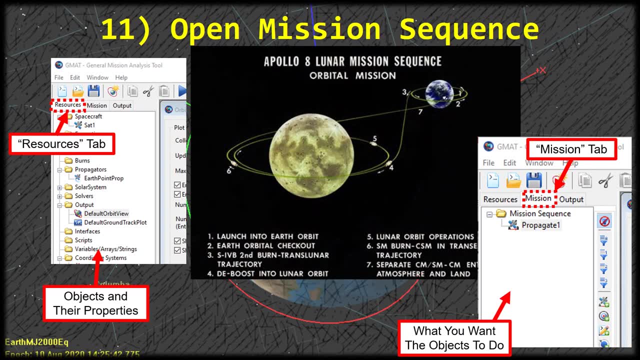 to switch gears and we're going to work on the mission tab and start specifying what we want the objects to actually do. But first let's start with an example. Right here I have a picture of the Apollo 8 lunar mission sequence. Apollo 8 was an orbital mission around the moon, So as you can see in this mission, 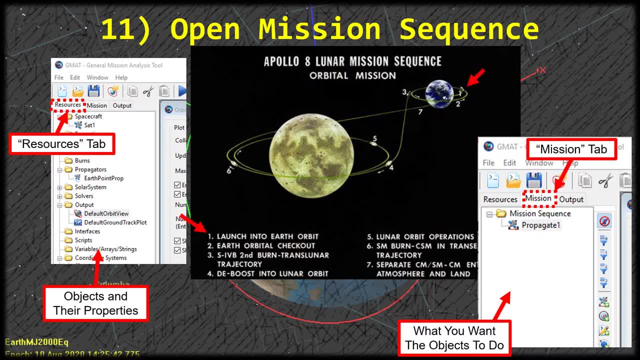 sequence. the first part is launching into the earth orbit And then from there there's probably going to do a burn to establish the earth orbit. It looks like number two there, Then on number three they do a burn to go from a translunar trajectory, meaning from earth to the moon. 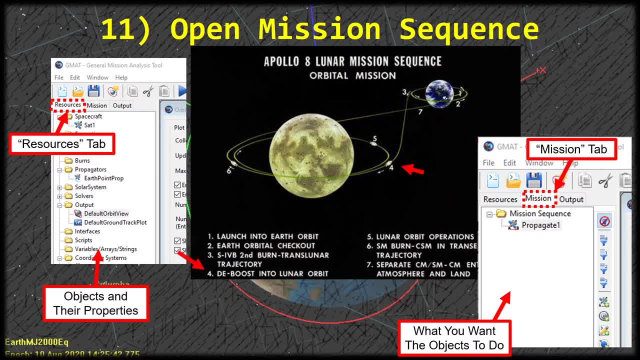 When they get to the moon they do another burn to go into a lunar orbit. Then they sat there for a bit and did whatever they need to while they were orbiting it. When they were done, they went ahead and went into another burn to leave the lunar orbit and head back to earth. That's number six. 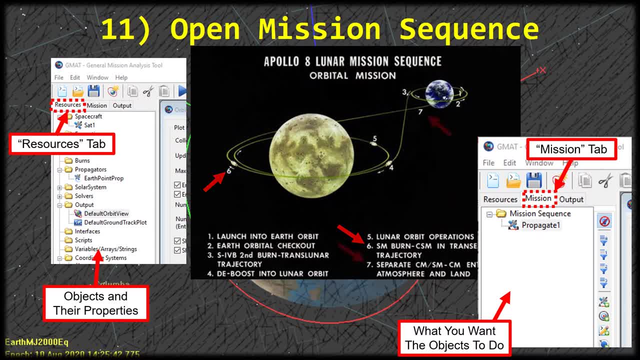 there And then, when they were getting close to earth, of course, on number seven is when they start doing their burns to re-enter the earth's atmosphere and land the craft. So, as you can see, by this mission sequence, they do a burn to go from a translunar trajectory, meaning from earth to the moon. 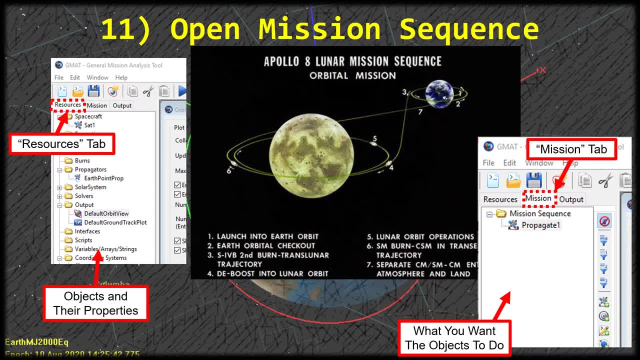 Really, there's multiple different, if you want to call them- orbits. there's different burns, there's different actions that are going on for the entire mission sequence, And so that's what we are wanting to do here on the mission tab is we're wanting to build all of these different. 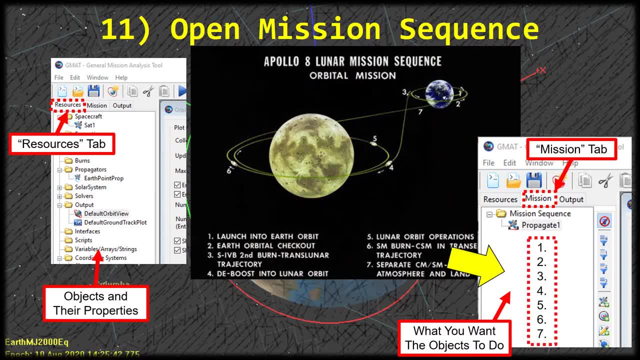 actions in the proper order so that when we simulate our project we get the correct behavior from our spacecraft And so from our example. it shows seven different events in the mission sequence. If we're going to do a burn to go from a lunar orbit, we're going to do a burn to go from. 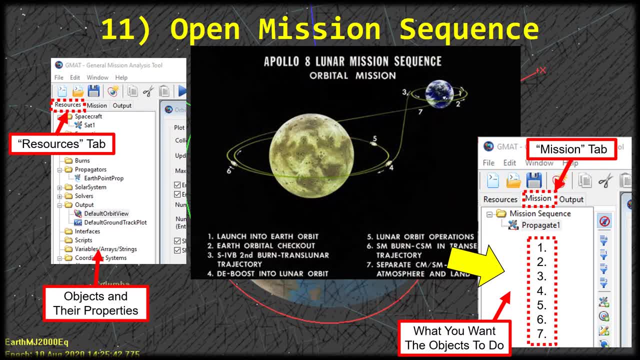 a lunar orbit. If we're transferring that over into GMAT, we'd have seven different items here in the mission sequence in order to try and build out that Apollo 8 lunar mission, And maybe we'll do that for a future video, just as a tutorial. that'd be pretty fun. So go ahead and click on the mission tab and 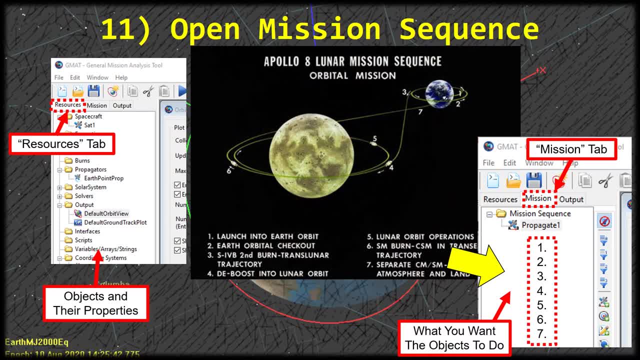 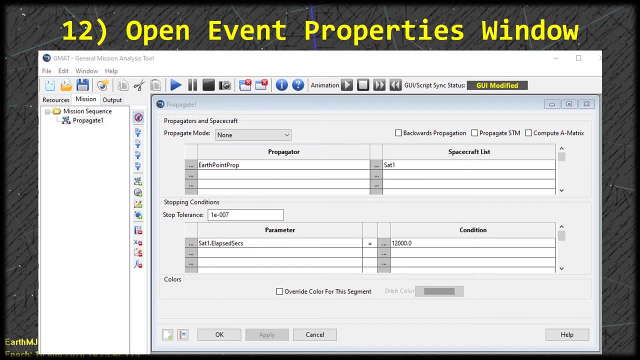 let's start building out our mission sequence. So let's go ahead and start editing the mission sequence in our simulation. The default simulation already has an event in there called Propagate 1.. Let's go ahead and double click that to open up the properties window. And when 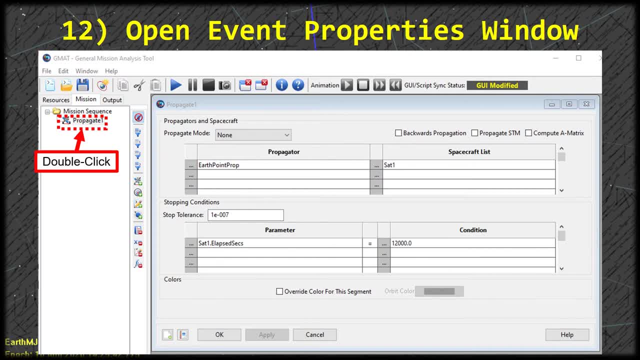 you'll do that. you'll see a couple things in here. You'll see in the spacecraft list what object the event is for And with its propagator you'll see how it's going to move that object And then towards the bottom you'll have the list of stopping conditions. The way that it works is: 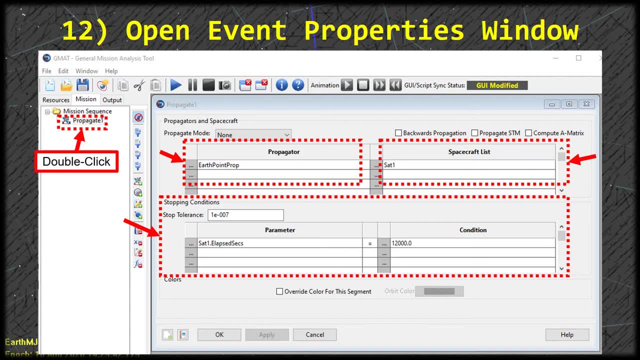 that if any of these become true, it will stop that event and move to the next event in your list. So if you have a dozen different stopping conditions, whichever one happens first is what's going to stop it and move it on to the next event. Then, if you look at the bottom, 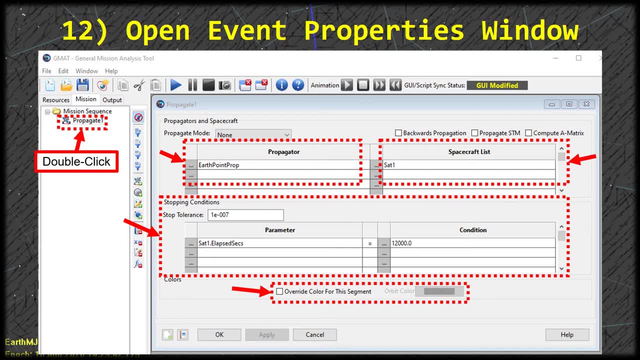 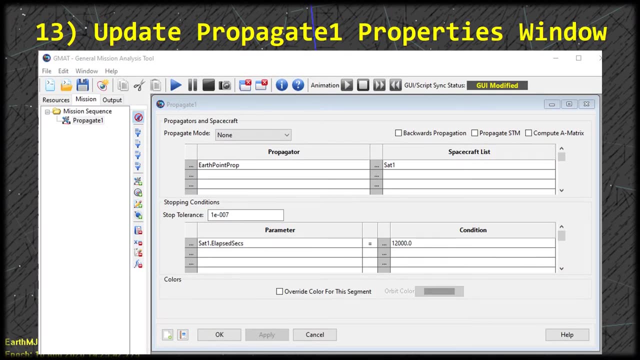 you have an option to override what color is plotted in the orbit view, And this is helpful when you have multiple events. You can see what those events look like compared to other events in your mission sequence. So let's go ahead and start updating this event for our tutorial using 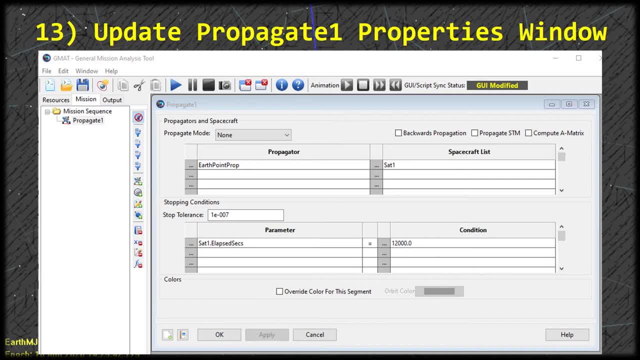 Sat1.. We're going to go ahead and change the stopping conditions for this event. If you look, the initial stopping condition would be elapsed seconds with a value of looks like 12,000.. This would cause our satellite to orbit the earth using the earth point prop for 12,000 seconds, until it. 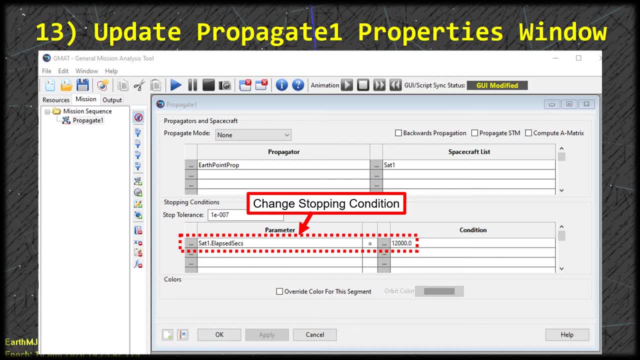 would stop and move on to the next event. What we're going to do is we're going to change the stopping condition. To do that, let's click on these dots to the left of the parameter we want to use for our stopping condition, And when you click on those three dots it's going to open up. 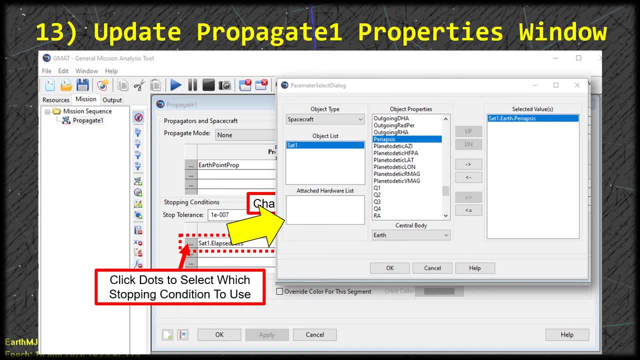 this dialog here, where it will allow us to choose the object and parameter for the stopping condition. Some of these parameters: you need to specify what the central body is. For instance, periapsis is the closest that the orbiting object comes to the central body, And so we need to. 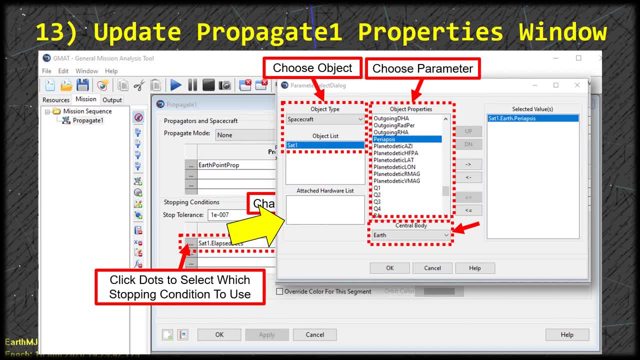 specify what the central body is, And then we're going to go ahead and change the stop and condition to what central body we're talking about. So on this sim it would be earth. So go ahead and make sure you select sat1 as the object and periapsis as the parameter that we're wanting to use as the 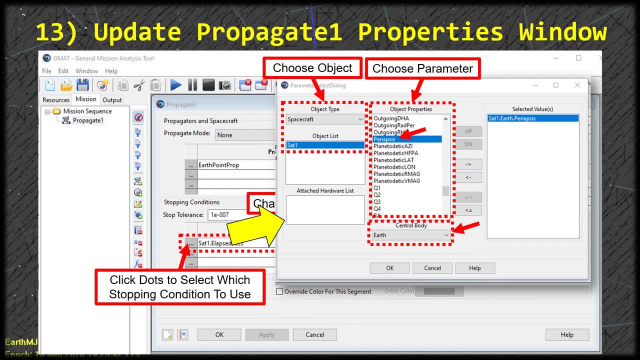 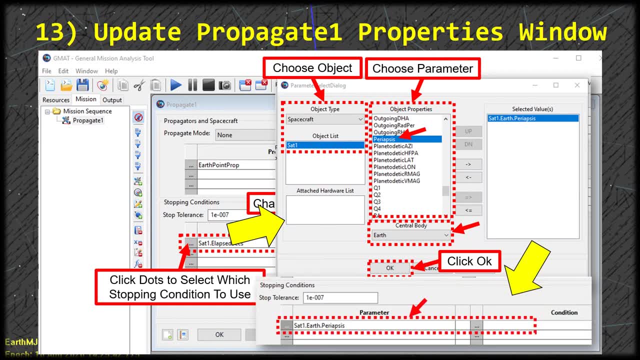 stopping condition And then use the right arrow to move it to the selected values And then go ahead and click OK. When you do that, you'll notice that the list of stopping conditions is updated and that periapsis doesn't have a condition to check for. This is because this particular 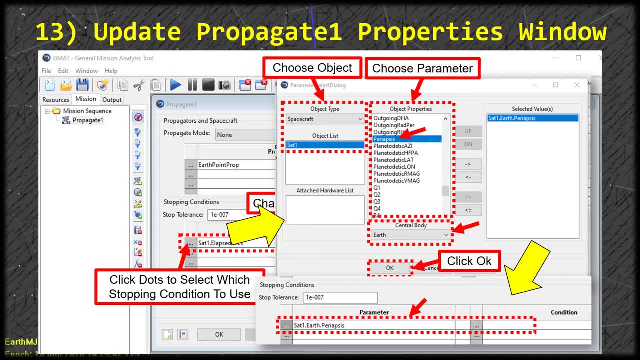 parameter is a location parameter, right. So that means that it will stop this event in the mission sequence when it gets to that location and then move on to the next event. So when you're done changing the stopping condition, click OK on the Propagate 1 properties window. 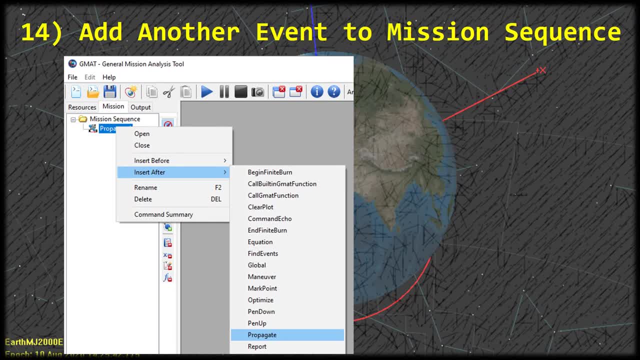 For this simulation, we're going to actually add another event to our mission sequence. If you right click on Propagate 1 and on the pop-up menu, if you choose Insert After, it will give you a list of different events that you could choose. Go ahead and find. 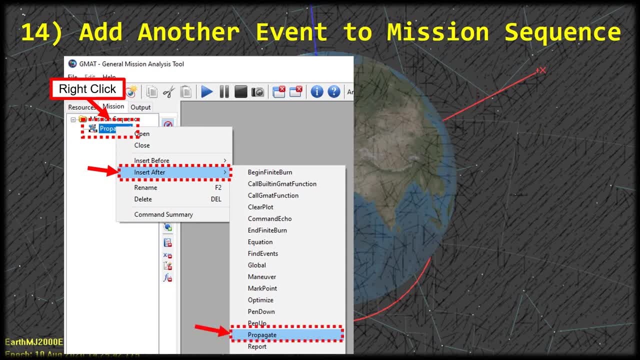 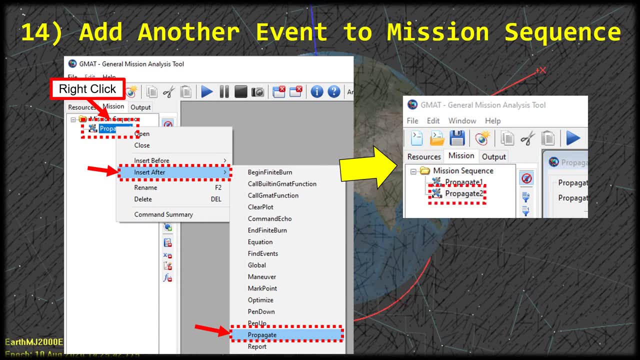 Propagate down there towards the bottom and click on it. When you do that, you'll see that in our mission sequence a second event has been added, called Propagate 2.. So the way this mission sequence is going to work is that it will run Propagate 1 until it encounters the first stopping. 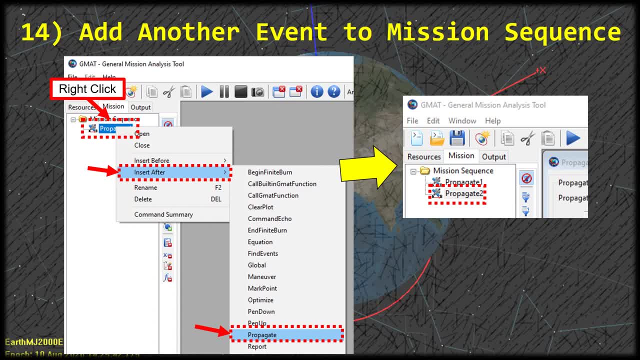 condition that becomes true, And then we'll run the Propagate 2 event until it reaches its first stopping condition. And then we'll run Propagate 2 until it reaches its first stopping condition. So let's go ahead and double click on that Propagate 2 and update its stopping condition. 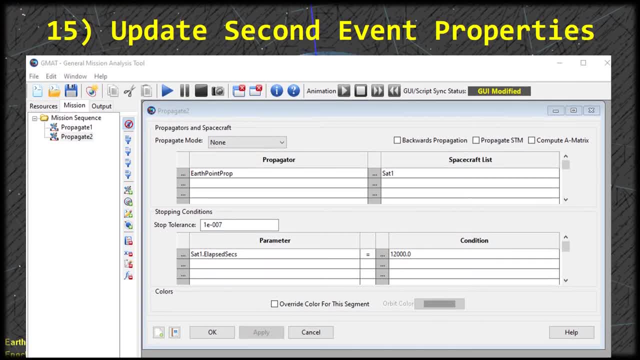 and properties. When the property window opens for the second event, again you'll see that it chose the Spacecraft Sat 1 and Propagator Earthpoint prop. So it's going to move the Sat 1 using the Earthpoint prop, which is what we're looking for And the default stopping. 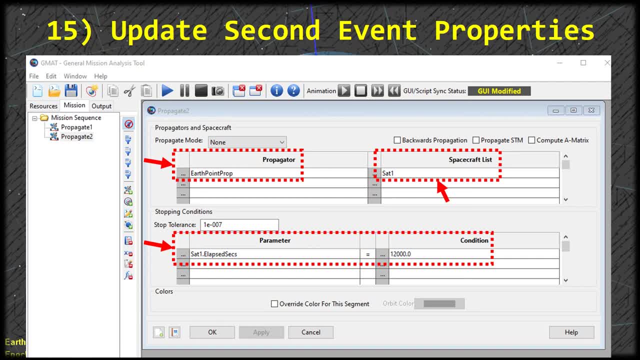 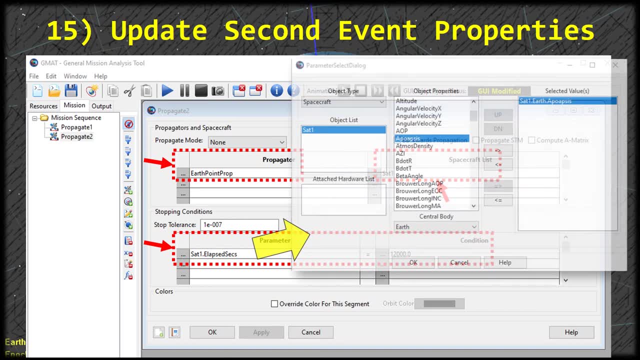 condition again is Elapsed Seconds, and that's what we want to change. So go ahead and click on those three dots to the left of Sat 1 Elapsed Seconds, and that will open up this dialog. For the second event, we're going to choose the stopping condition as the location of Apoapsis. 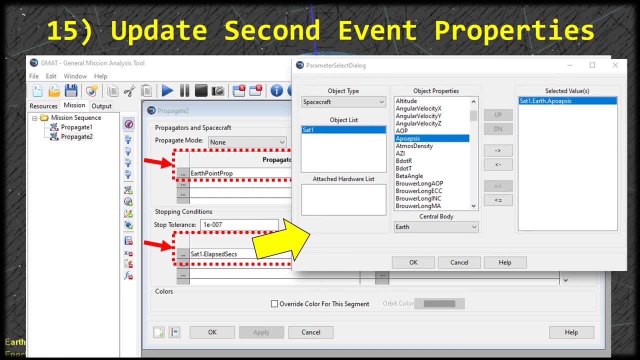 So, in the object we're wanting to create the stopping condition, we're going to choose Sat 1.. We're going to scroll down Object Properties to find Apoapsis And again, since this is a location of which the satellite is furthest from the body it's orbiting, in this case, 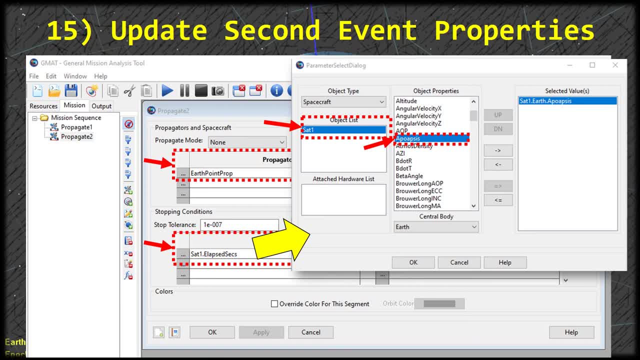 the central body. we need to specify what that central body is for the stopping condition, which is Earth. So make sure that says Earth, Then use the right arrow to pass that parameter to the selected values we want to use as a stopping condition. If there's anything else, 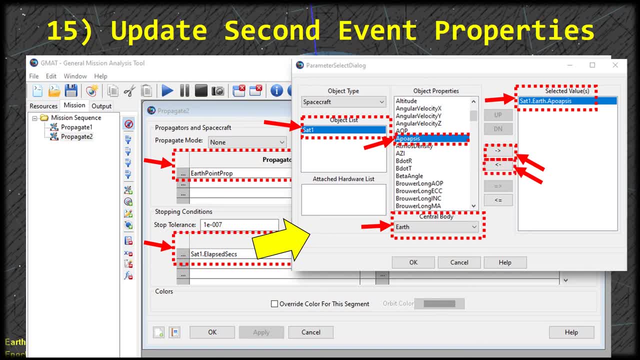 in that selected values. use the left arrow to remove it from the list. Then, when you're done with that, click OK And you'll notice in the list of stopping conditions that it changed from Sat 1 Elapsed Seconds to Sat 1- Earthpoint Propagator- Earthpoint Propagator. Earthpoint Propagator. 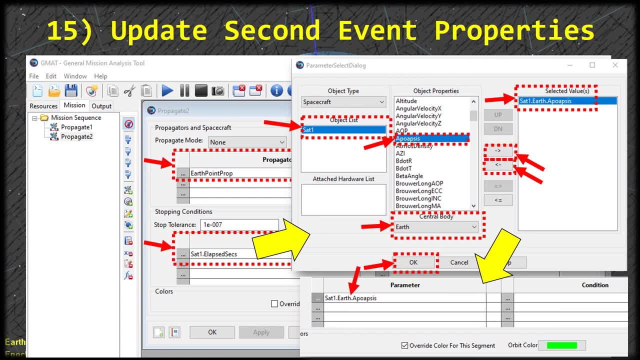 Apoapsis And since it's a location, there is no stopping condition. Just whenever the satellite gets to that location, it's going to stop, And in this one, just for this tutorial. so we can see the difference between the two events and how they work together, I went ahead and chose. 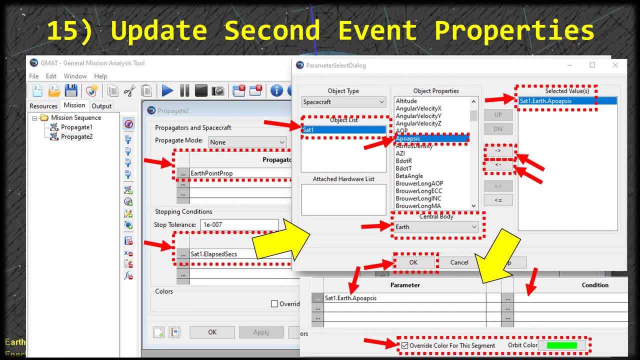 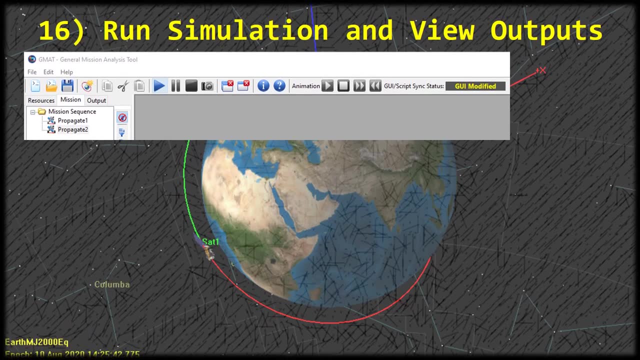 to override the color for that segment and make it bright green And then go ahead and click OK on this Propagate 2 window to save the changes that we made to this event in the mission sequence Autoproperties. All right, we're done making changes and updating both the objects and the events that we want to. 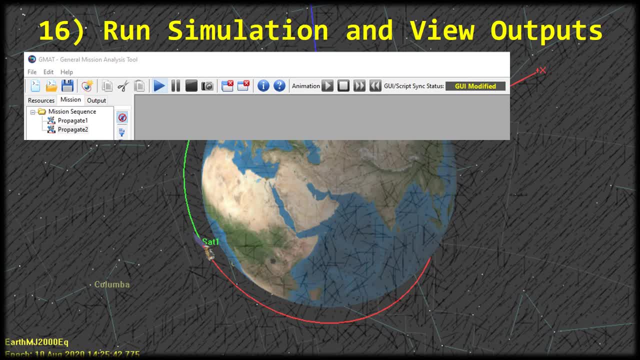 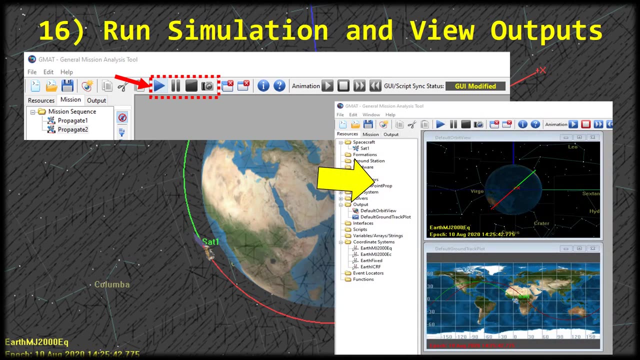 occur. And so now comes the point where we want to actually run our project, to simulate the mission sequence. So to run the simulation, you have the buttons here in the toolbar. You've got the play button. There's the pause button and stop button, And so if you hit play then you'll notice that. 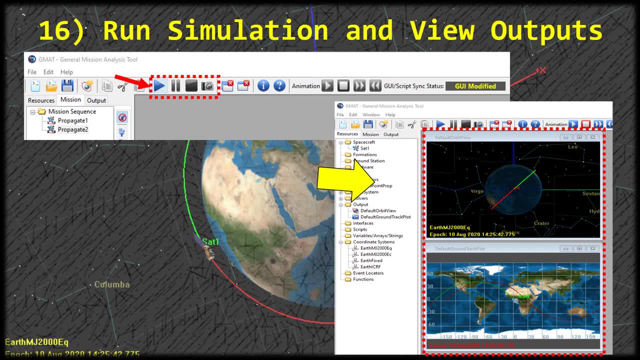 these two windows appear inside of the workspace area And those appear because we had them in the outputs folder right. We had a default orbit viewer that we just did the properties for. Then we had the default ground track plot. After this simulation has finished running, we're actually. 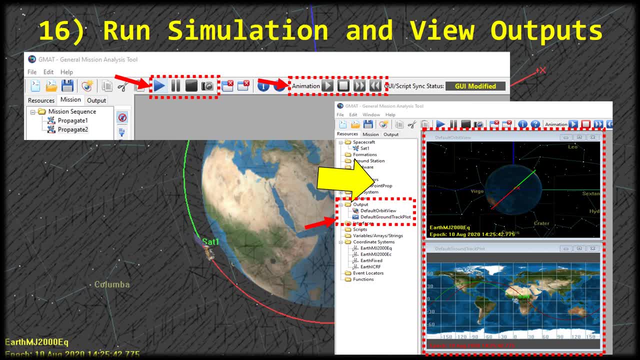 able to animate the results, to see the satellite travel over the ground track plot or to see the satellite orbit around the earth, to visualize the mission sequence. And we'll check that on the next slide. But real quick, there's also here on the top right this GUI modified. This simply means 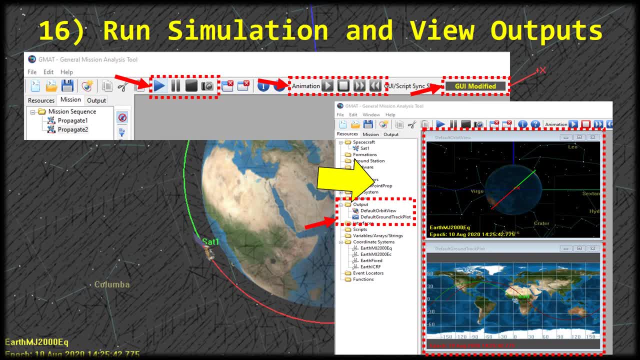 that you have the script file using this GUI, but you haven't saved it yet. So before you close out of any of this, after you're done checking out the results, make sure that you save it if that's what you're wanting to do. So I went ahead and made the orbit viewer bigger and I'm going to click the. 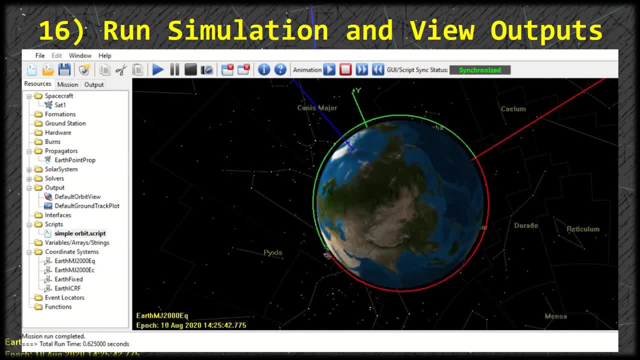 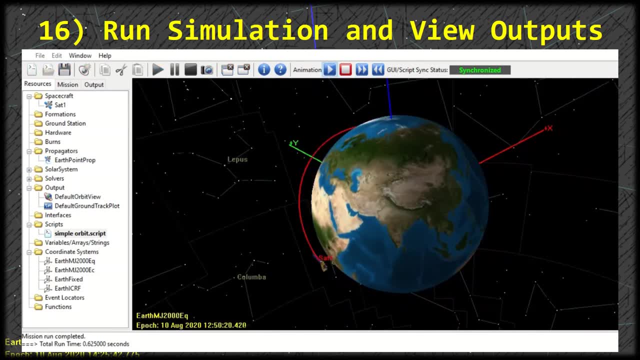 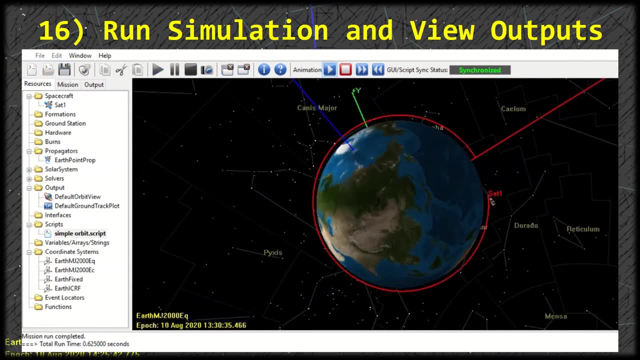 animation button a couple times here so that you can see the satellite moving around the earth. I'll go ahead and pan it and rotate to get a better view of the orbit and click animation again. So, as you can see, this is the first event And then when that event hits its stopping condition at periapsis, 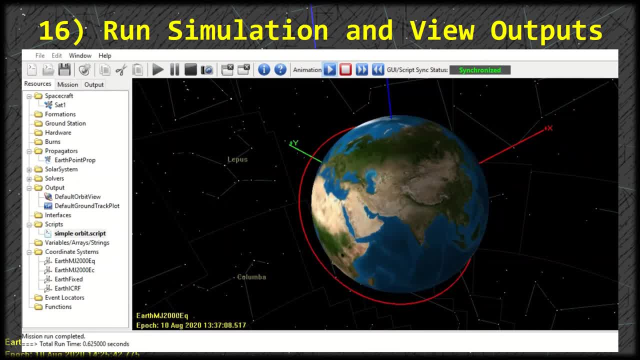 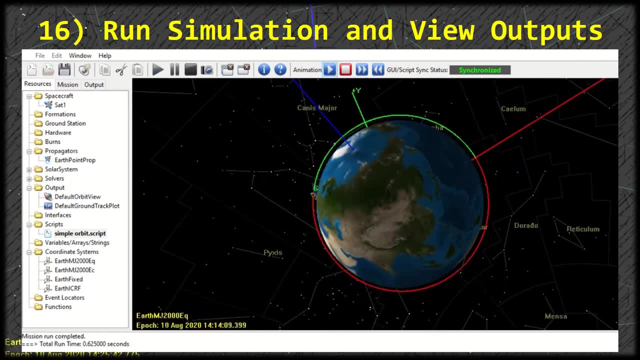 the second event starts and that's where we're getting that green line that goes to apoapsis, And of course I can zoom in closer. I can zoom out just to get a better shot not only of the orbiting object but also the object being orbited. So this is pretty cool. 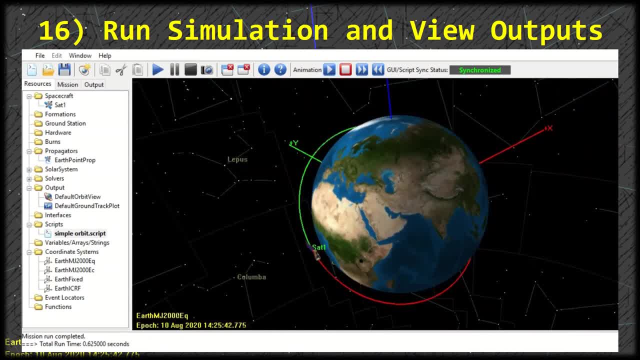 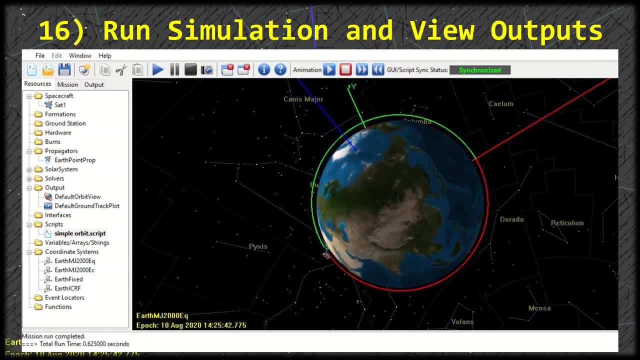 Go ahead and play with it and check it out. And that's where I'm going to end it for this video. If you liked what you saw and you want to see more of this, please subscribe to my channel. If you want to see some more like comment, subscribe. I'll see you in the next video.